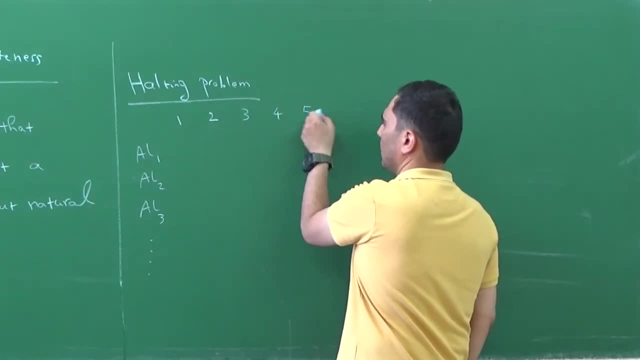 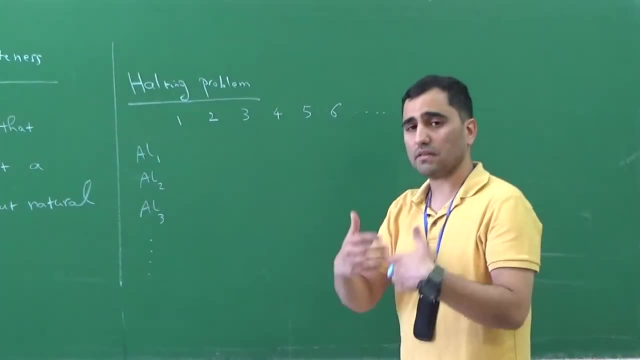 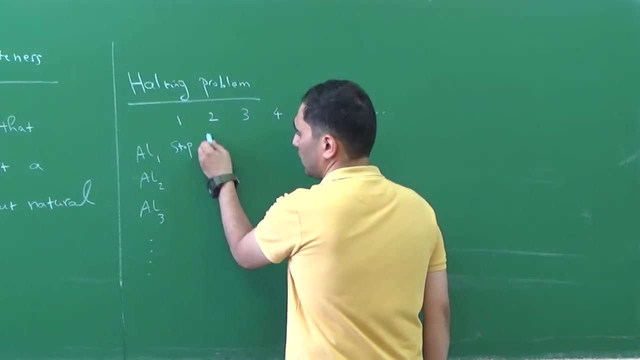 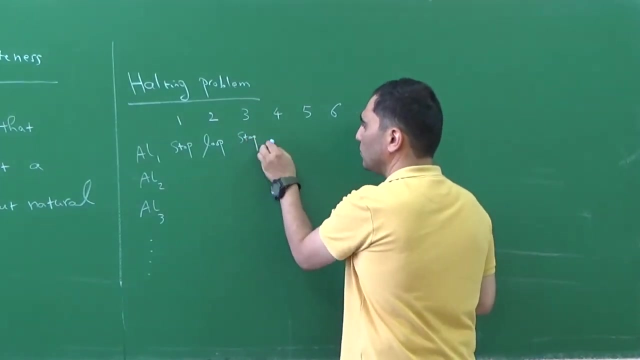 As an input. So one, two, three, four, five, six and so forth. When I give a natural number as an input to each of these algorithms, the algorithm starts to work and it may happen that my algorithm stops or gets into a loop. So I have a table of stops and loops, So each 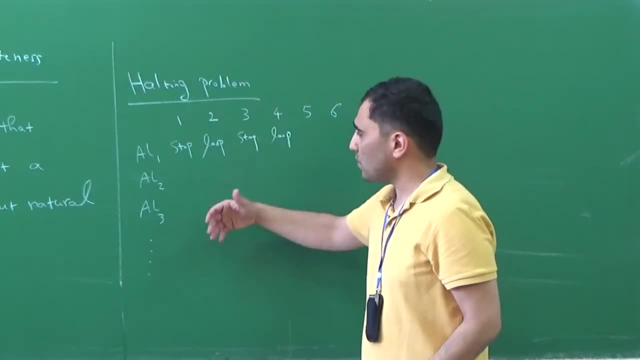 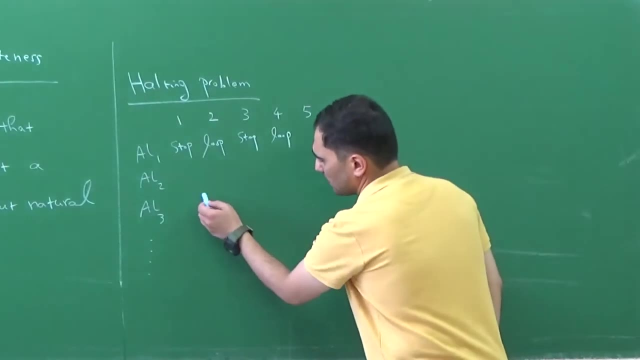 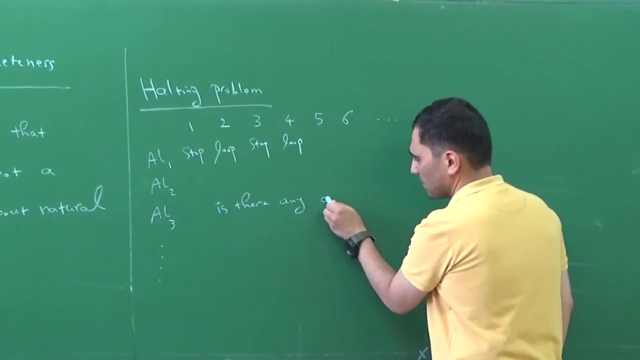 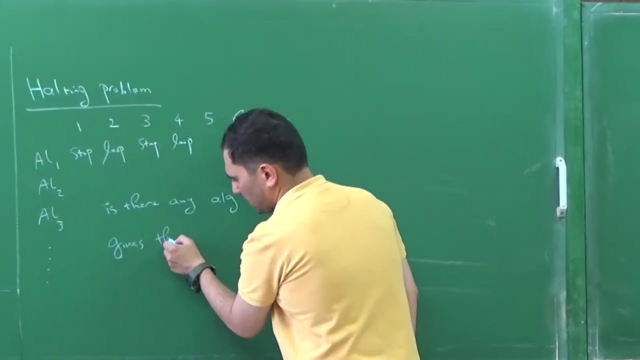 of these algorithms. given a natural number, It stops or gets into a loop and I have a full table of that. Okay, the halting problem says: the halting problem is the following: Is there any algorithm that gives this table? 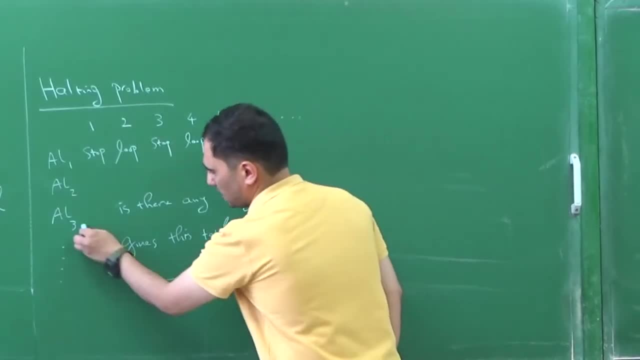 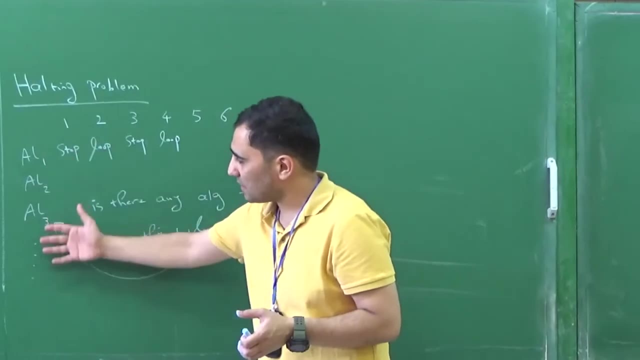 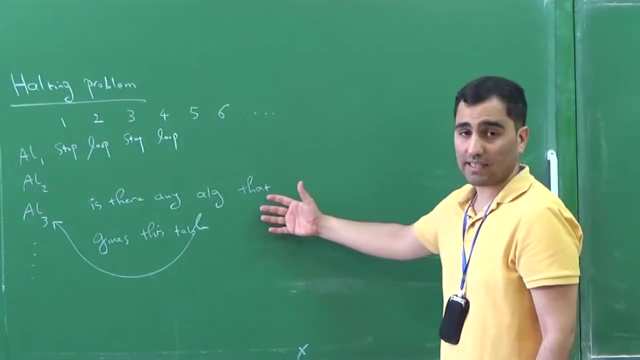 This table, And I mean this table. So the question is: is there any algorithm that can tell you whether or not any of these algorithms stops at any of these inputs? Alright, The answer to this question is negative, and I'm explaining here why. Okay, so the 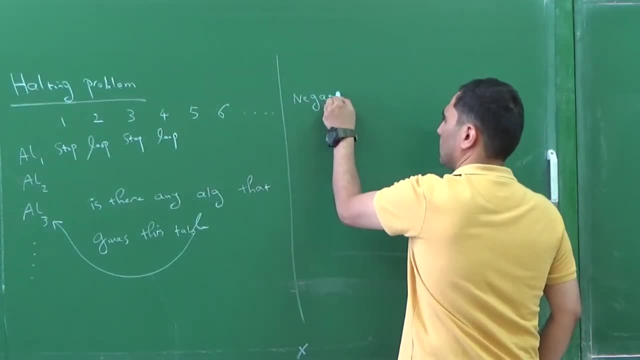 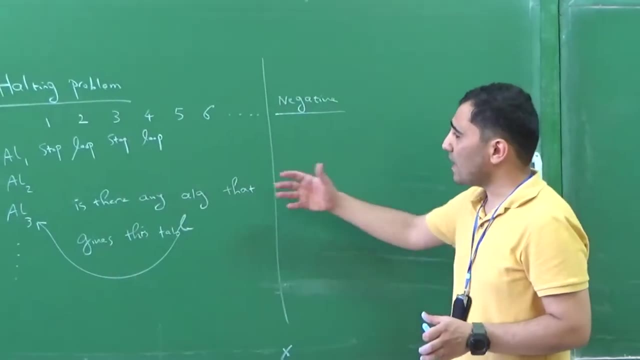 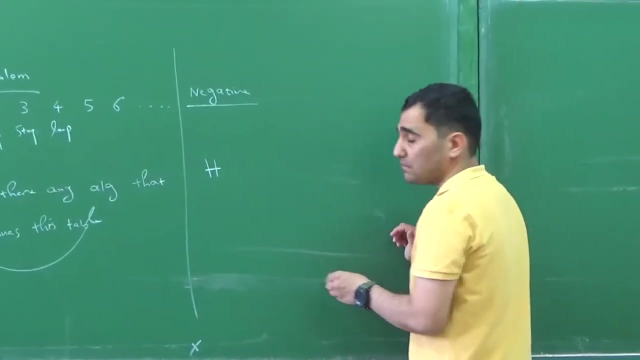 answer is negative. Negative, And the reason is the following: If you have such an algorithm that can give you this table, then you may have this algorithm that I'm writing here. algorithm H- H gets a natural number as an input and does the following: Okay, if algorithm 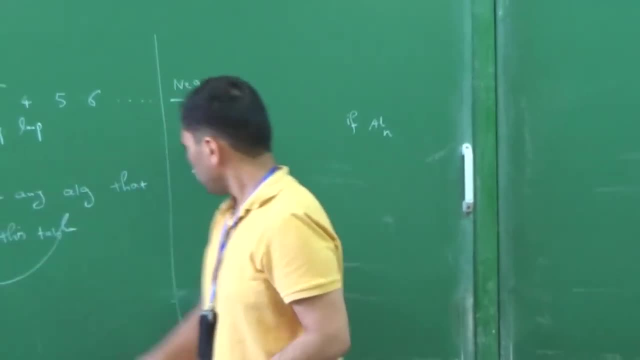 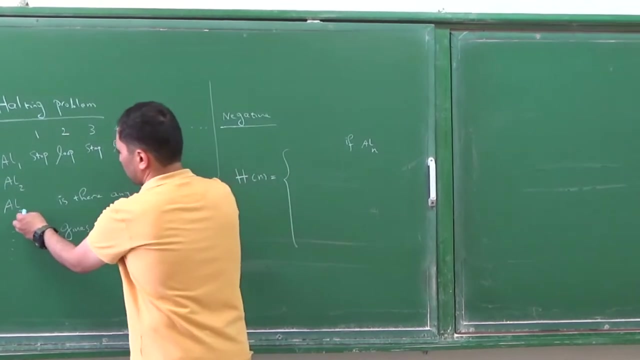 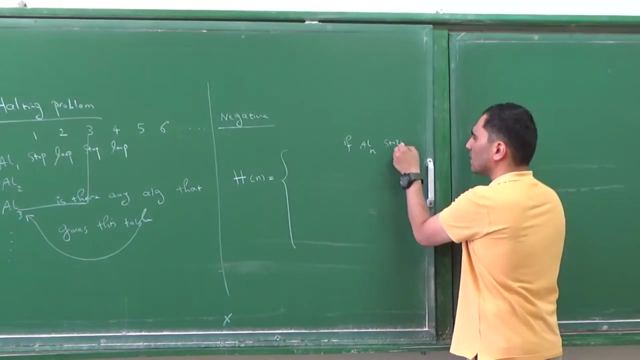 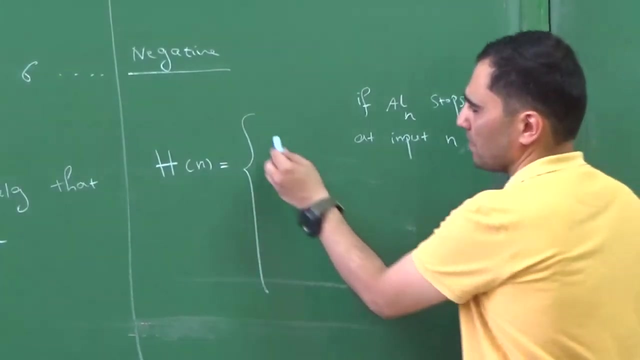 number n here. so when you give a natural number n as an input to my algorithm H, it just looks at algorithm n and input n, for example algorithm 3 and input 3.. So if algorithm n stops at input n, then H does not stop, It just gets into a. 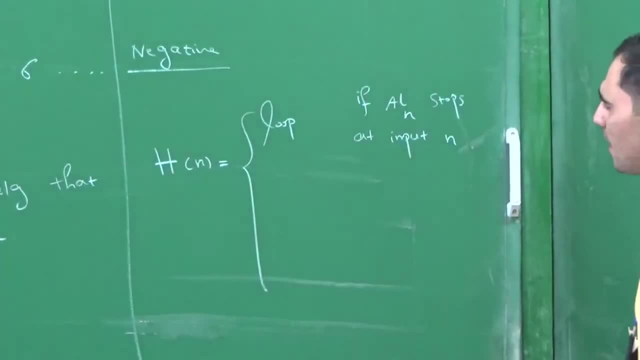 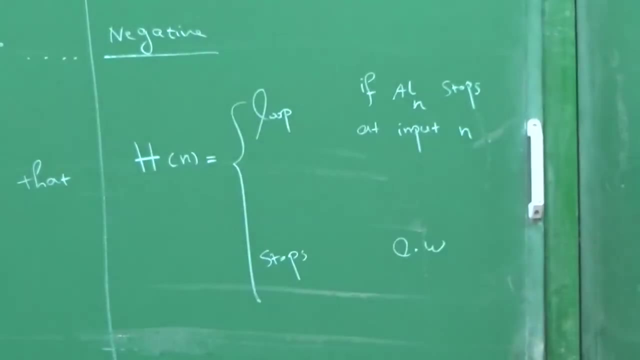 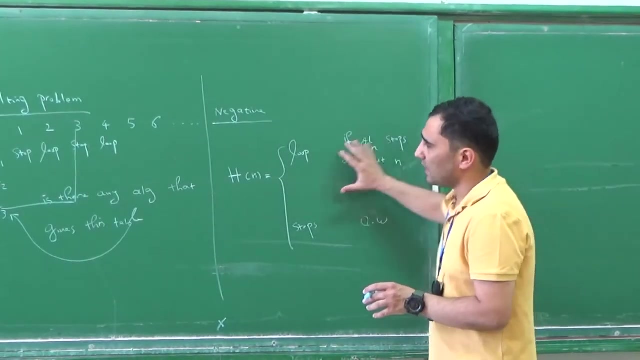 loop. You may just put the loop yourself here And otherwise my algorithm stops. when n is given as an input. All right, You may convince yourself that H is an algorithm because checking this part is by looking at this. assumed term is safe. And if you putening, H is an algorithm too. and as an input, the H widow itself an algorithm which will pay more. e Dualization should be able to transit. so you see, we see next, but this one is the algorithm. right. Then I have to say here you take, H is an algorithm because checking this part is by looking at this. 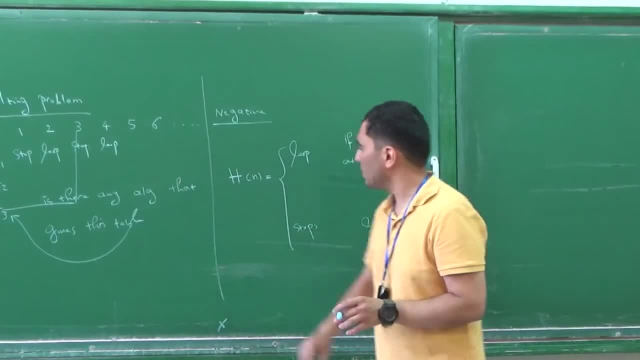 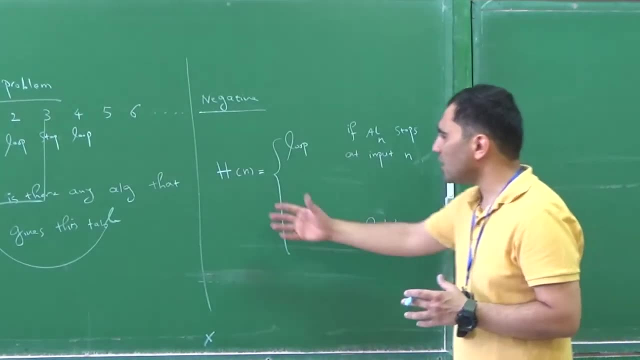 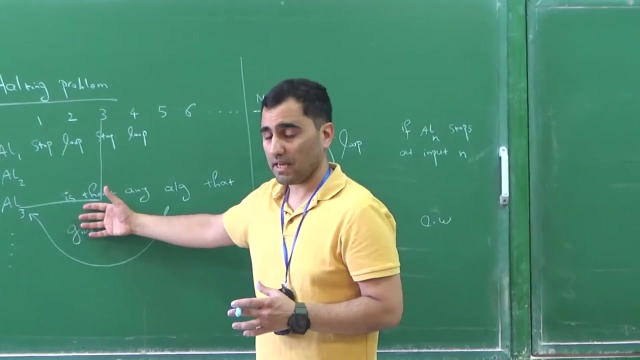 table, and this table itself is given by an algorithm, So what I have written here is a valid algorithm. Okay now, on the one hand, H is an algorithm and it's supposed to be in my list, because I said I have listed every single algorithm here, So H is one of the. 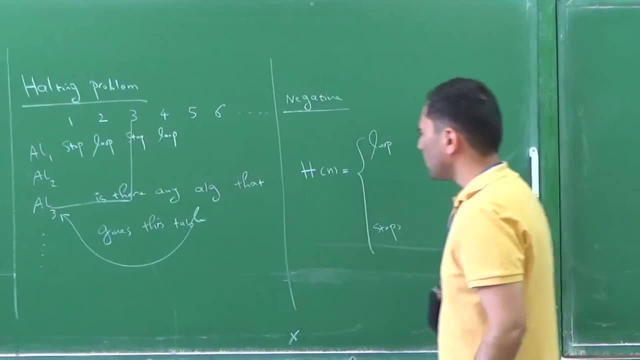 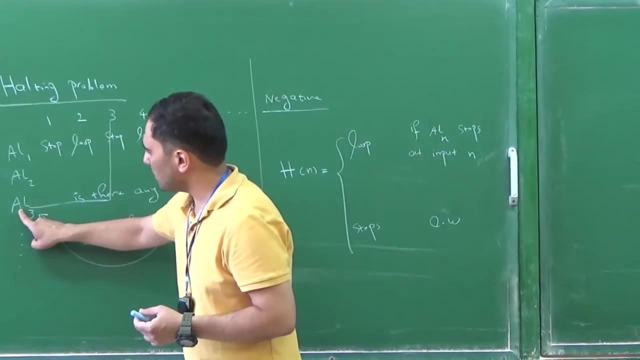 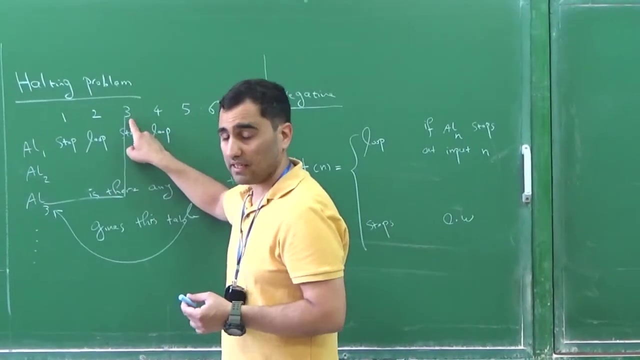 algorithms that I have listed here, But at the same time, H is different from everything that I have listed here because, for example, H is different from algorithm 3 at input 3.. It does the opposite thing as algorithm 3 does at input 3.. And H is different from algorithm. 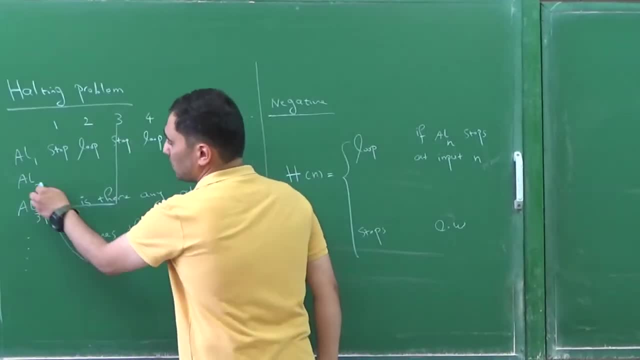 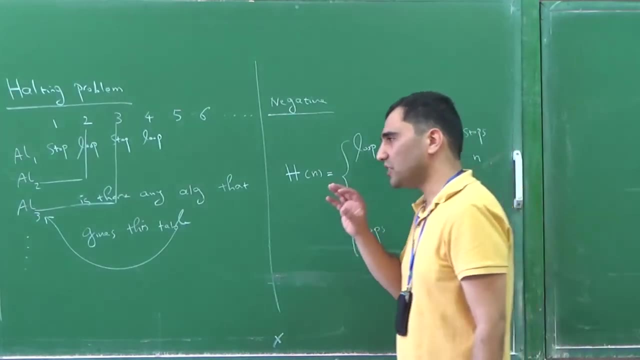 2,. sorry, H is different from algorithm 2 at input 2, and it's different from algorithm n at input n. So on the one hand, H is in my list and, on the other hand, H is different from everything that I have listed, and that's a contradiction. 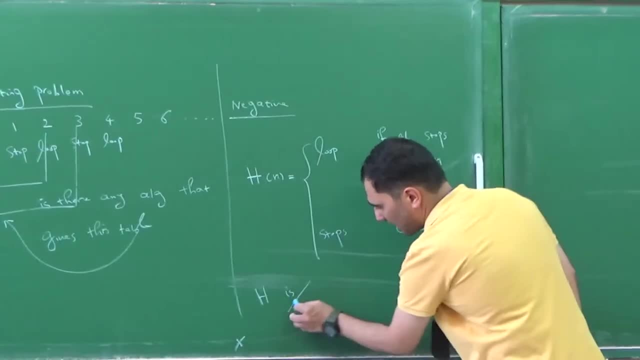 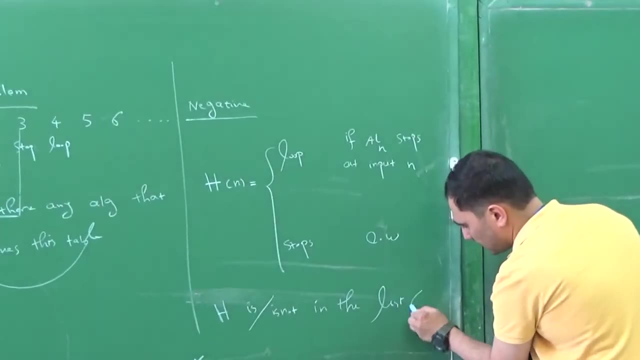 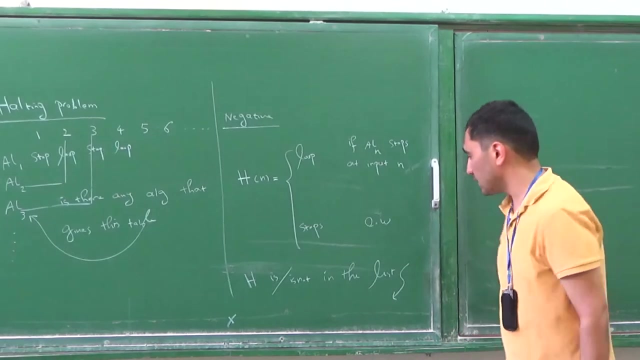 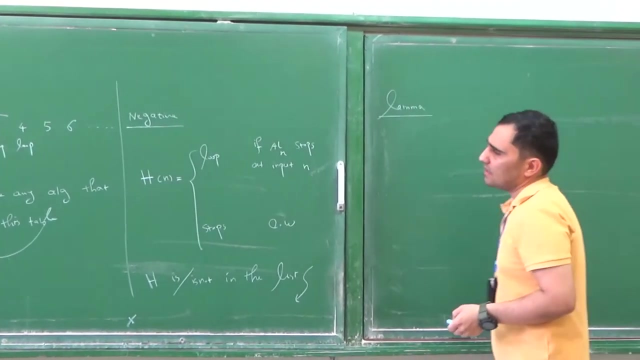 So H is and is not in my list and that's a contradiction, Alright. so what does this have to do with the question of decidability in mathematics? The connection question comes in this lemma. The lemma says: whatever the algorithms describe can be written with a first-order formula. 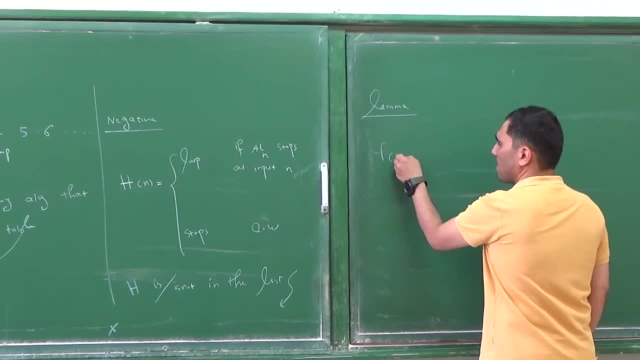 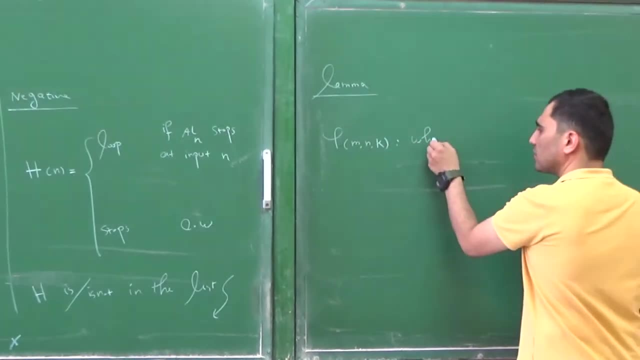 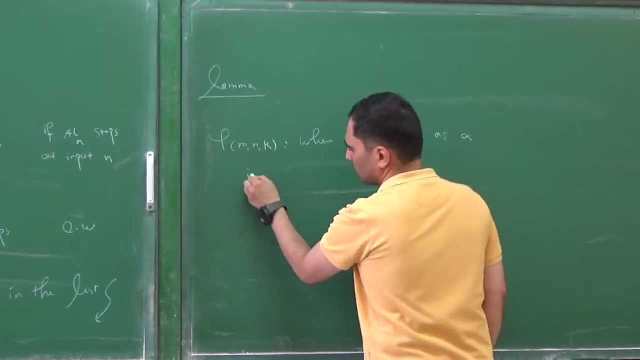 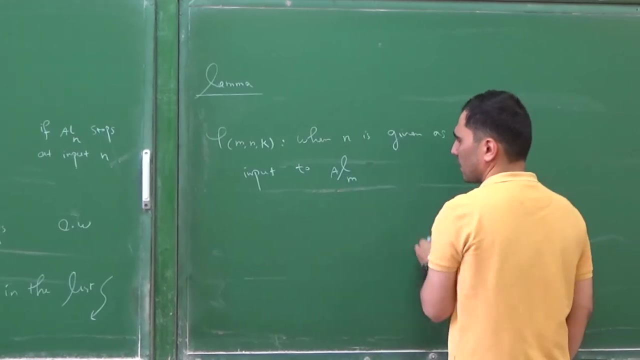 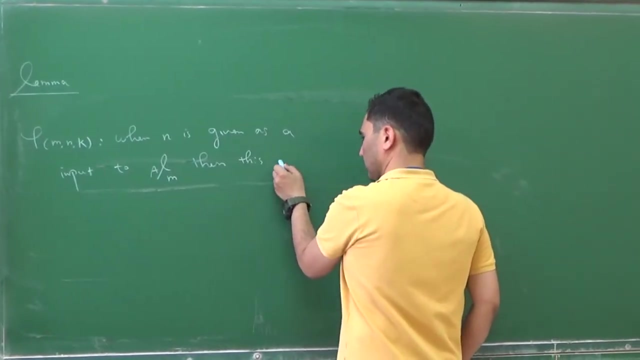 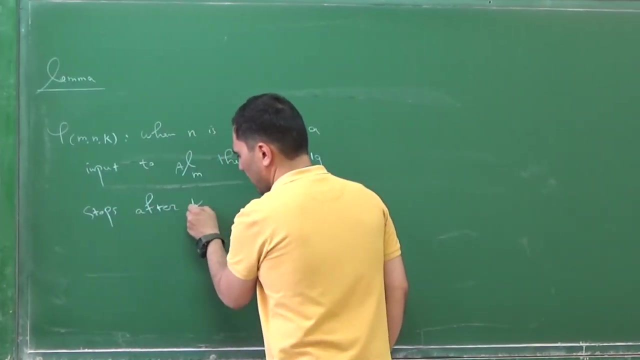 more accurate. There's a formula phi of m, n and k that says the following: When the natural number n is given as an input to algorithm number m- let's say algorithm m- then this algorithm stops. this algorithm stops after k steps or after running k. 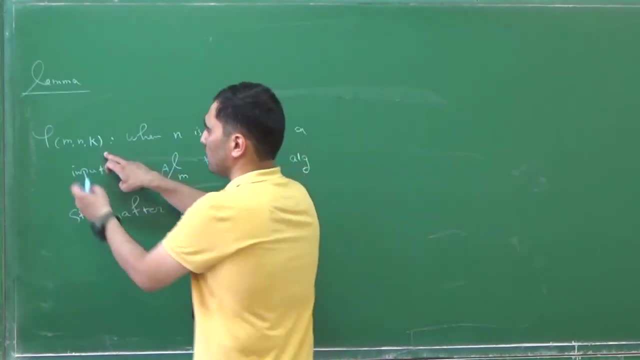 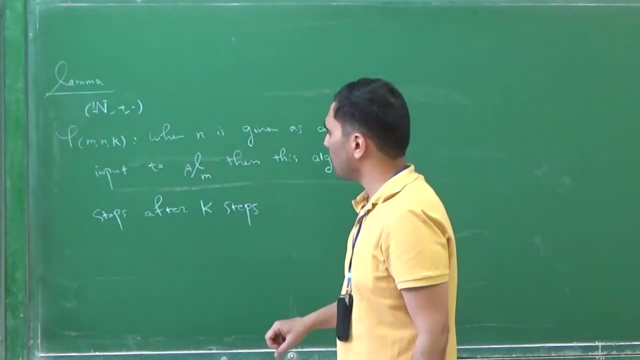 commands. So I have a first order formula. This first order formula is written in this structure. So this is a formula written in the language of addition and multiplication and says: when you give n as an input to algorithm number m, it starts to work. 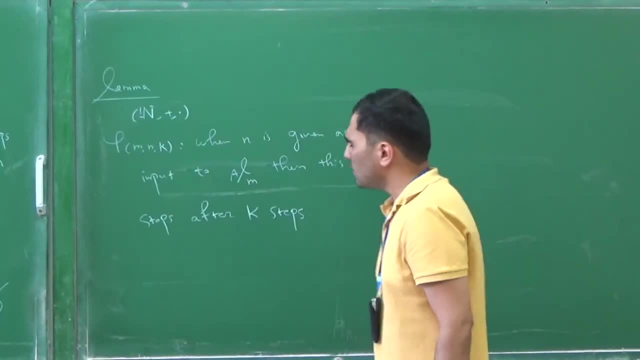 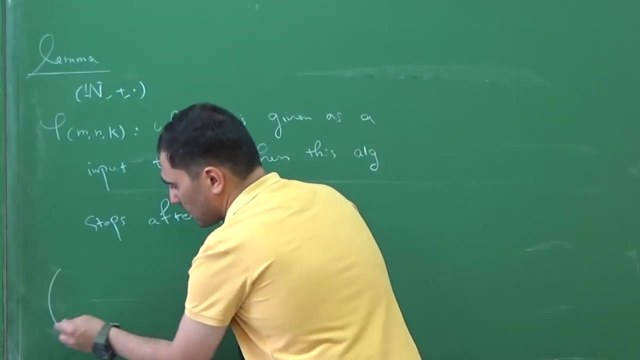 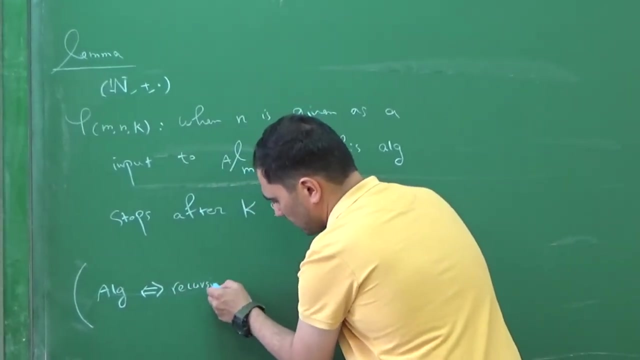 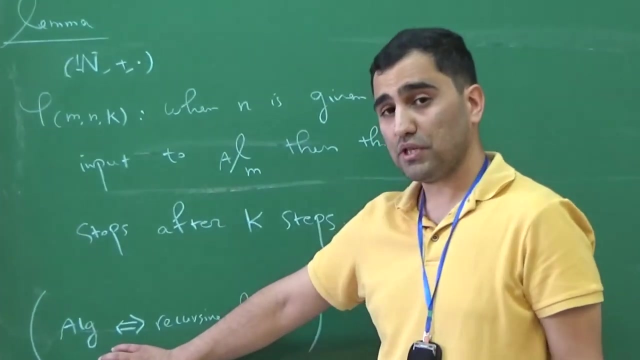 and it stops running k commands. So why is it possible to write such a thing as a first-order formula? The reason is that the concept of algorithms is connected to the concept of recursive functions, and this connection is called Church's thesis. Whatever you can compute using computer algorithms can be done. 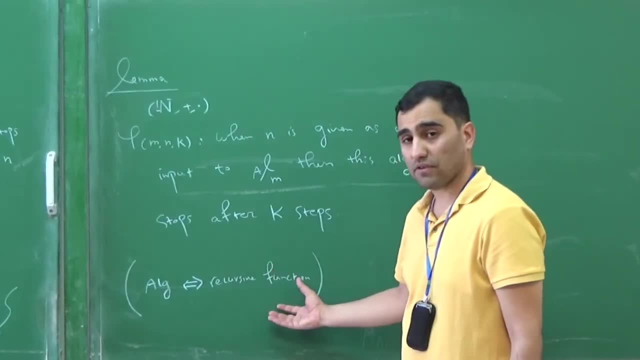 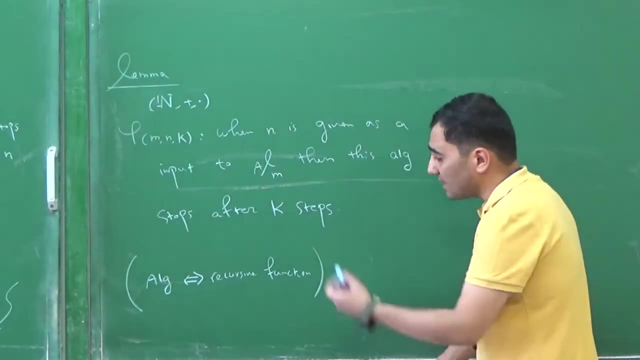 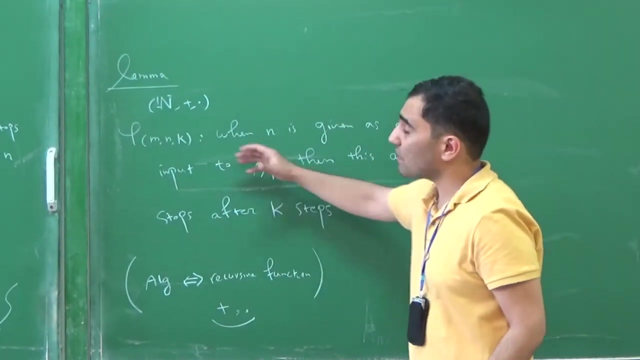 can be calculated via a recursive function, Recursive function. you may look for the definition of recursive functions, but they have an interesting recursive definition and you may prove that they are definable using addition and multiplication, and that's the reason that you can write this formula using only addition and multiplication of natural numbers. 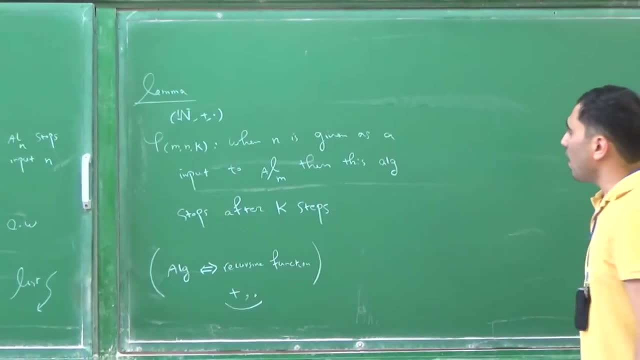 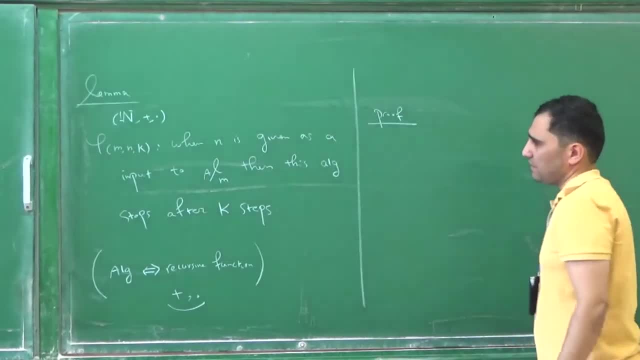 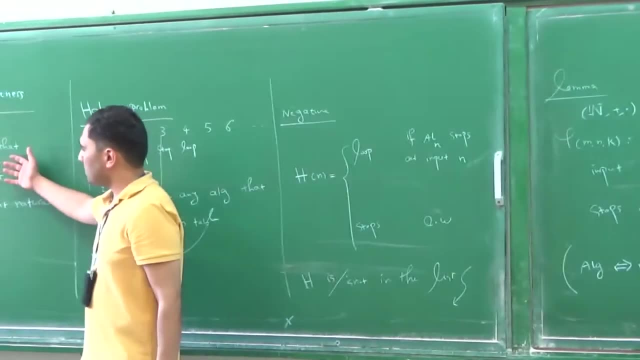 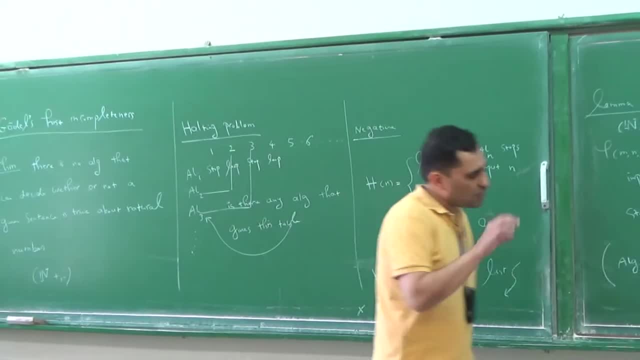 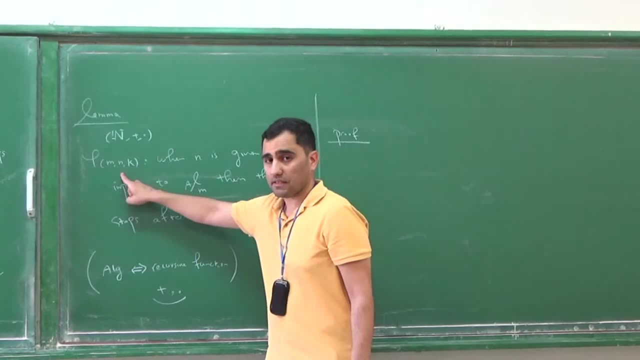 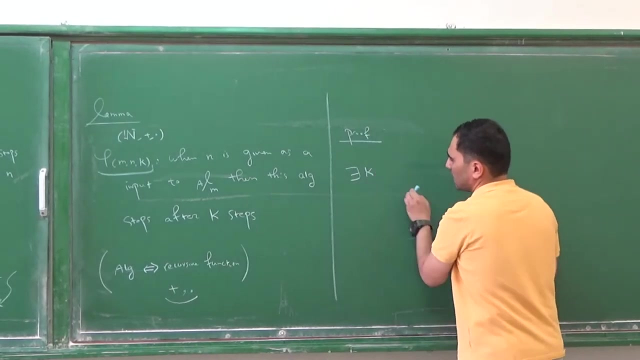 or not a given sentence is true about natural numbers. If you do have such an algorithm, then your algorithm should decide about such sentences as well. Alright, okay, let me just be more accurate. I'm just going to write a sentence here. Exist K such that 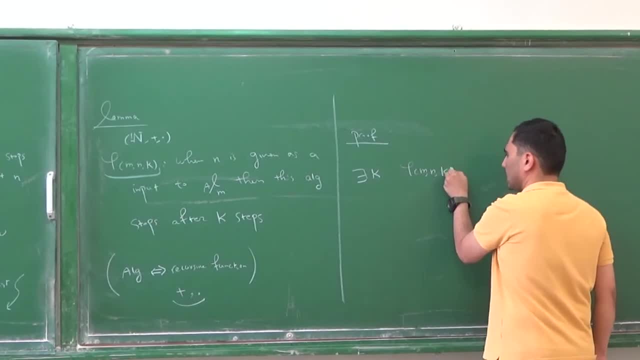 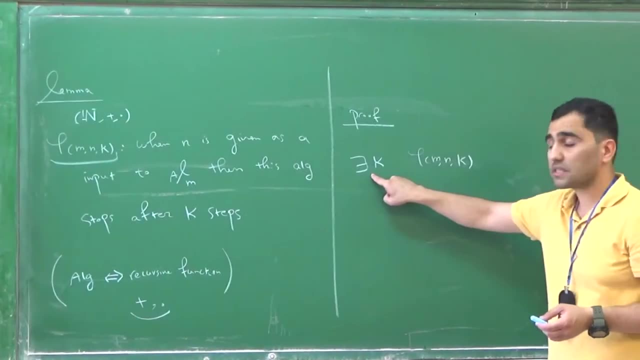 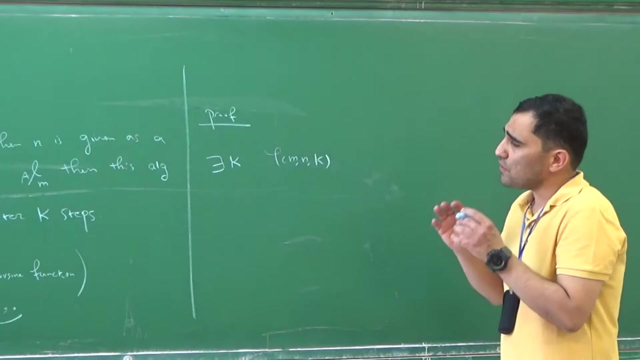 PHY of M, N and k. Look, this sentence says that when you give N as an input to algorithm number M, it stops. There's a final number of steps at which your algorithm stops. Alright, so if you have an algorithm that can, 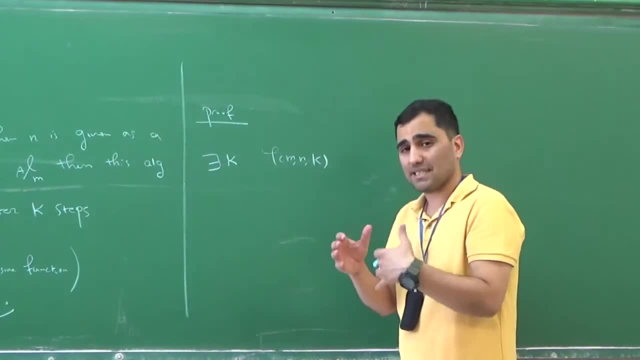 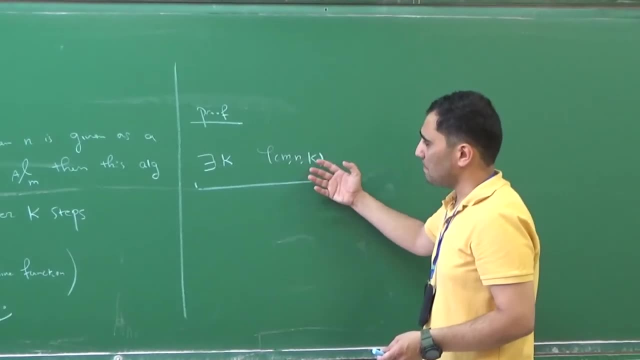 decide about natural numbers, that can decide about sentences about natural numbers. then it can decide about these sentences as well. But deciding about this sentences is a bit challenging. talk than earth行 is warm. This is just a good Burning Stones. okay, whatever to ask for. 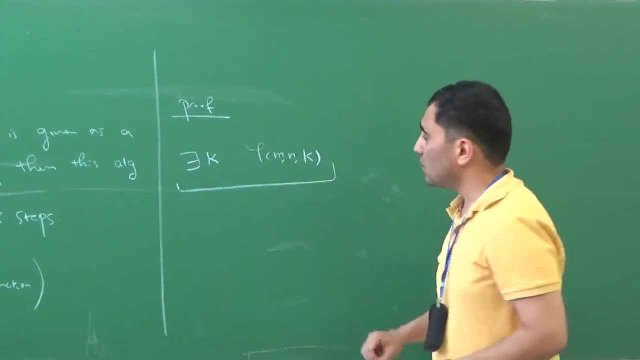 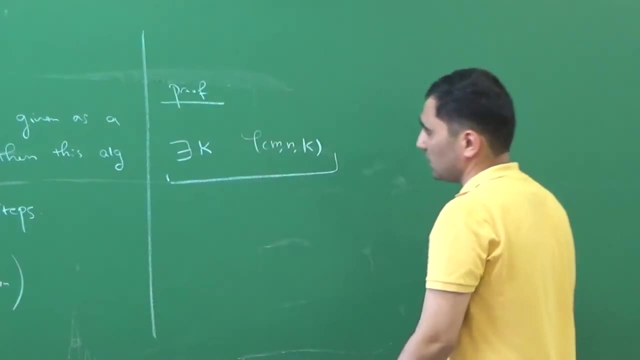 about whether or not algorithm stops at inputs. So if you have such an algorithm, then you have decided the whole thing. problem and that's not possible and that's a contradiction. So the proof is that if you do have an algorithm that can decide about sentences in natural, 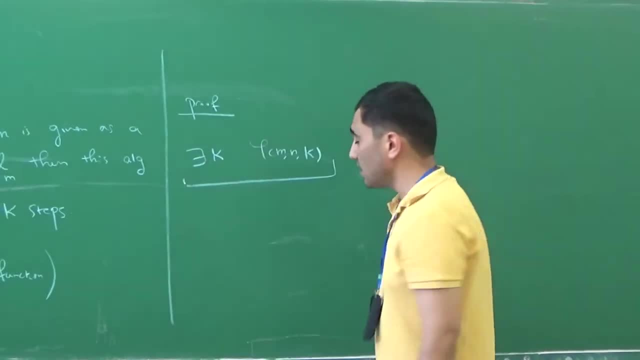 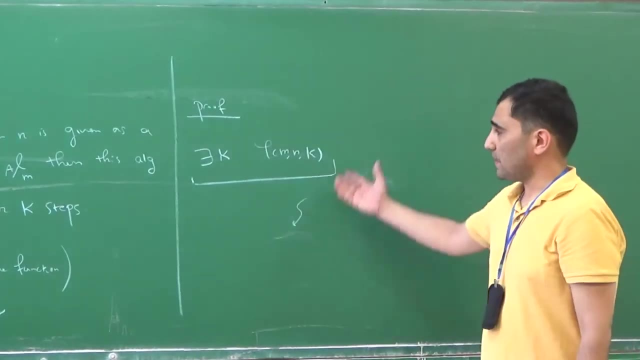 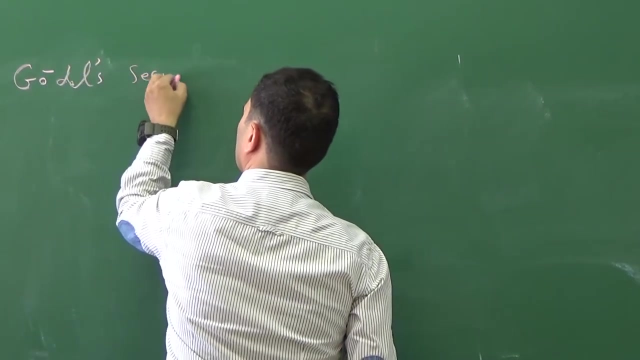 numbers. then you have an algorithm that can decide the whole thing. problem, and that's impossible and that's a contradiction. Alright, so now I'm going to talk about the second incubation theorem, but after wiping out these things. Second incubation theorem. 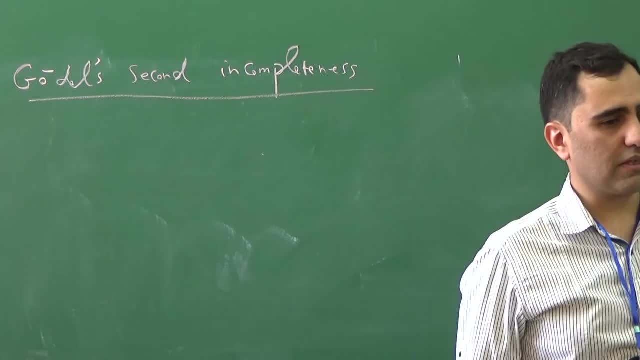 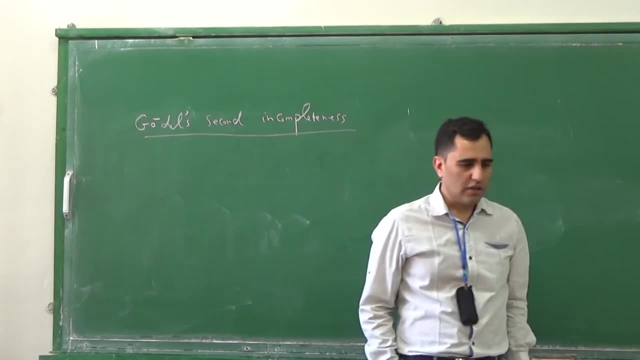 So remember that the first incubation theorem was about the question of the solubility of mathematics, but the second one is about the question of consistency of mathematics. You know, mathematicians use the set of axioms of mathematics and they start proving things. Is it possible? 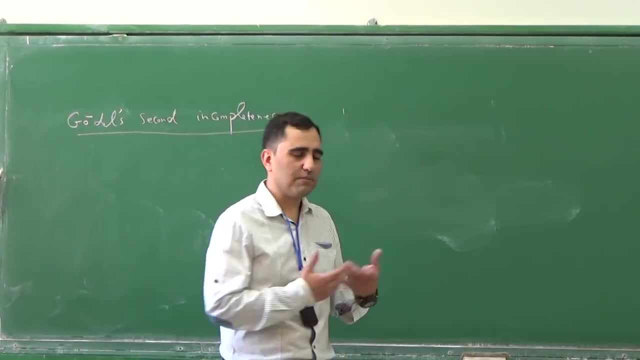 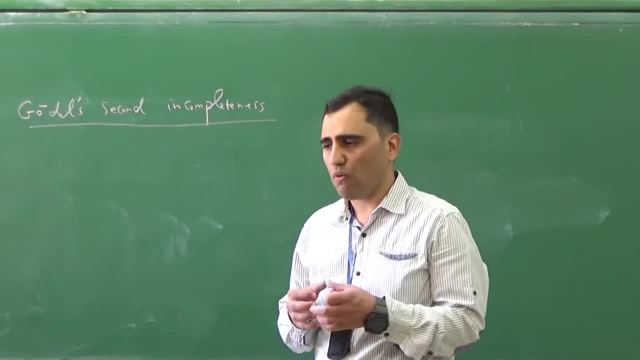 that I prove a theorem- 5 to 10?- And then at some later point, I prove the negation of 5.. So the question is that: is mathematics contradictory or is it possible to prove that it's not contradictory? I'm going to talk about ZFC. 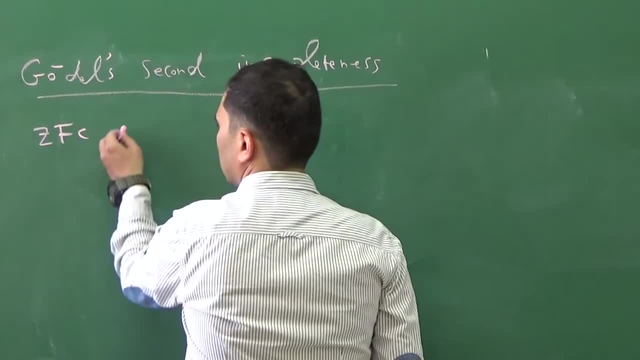 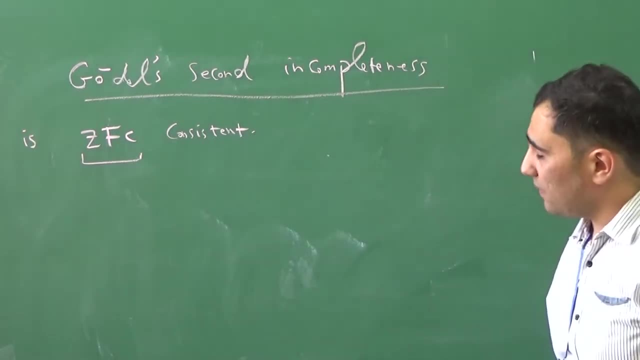 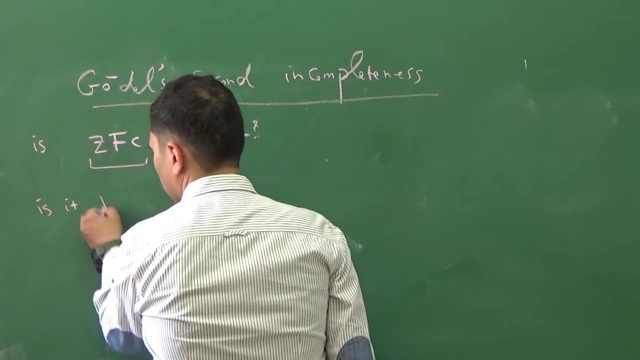 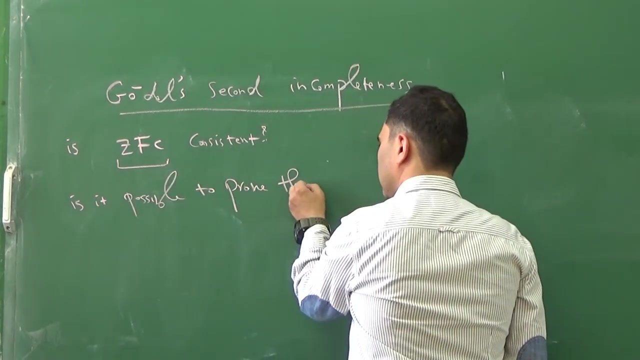 So the question is: is ZFC consistent? And ZFC is the set of axioms for the set theory. So the question is- let me just write it in a better way- is it possible? is it possible to prove that ZFC is consistent? 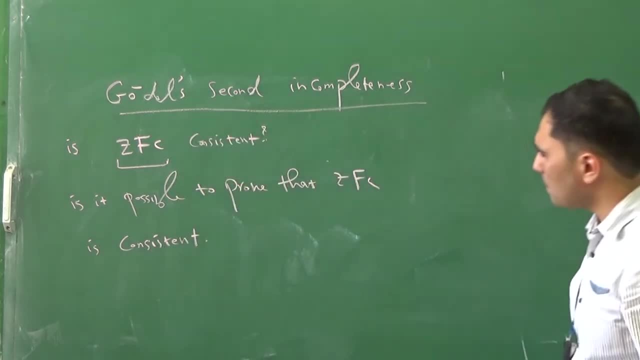 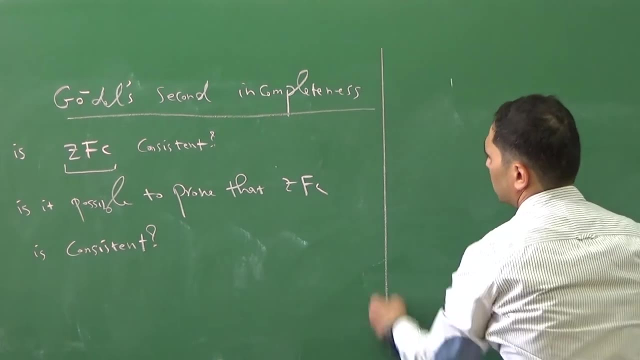 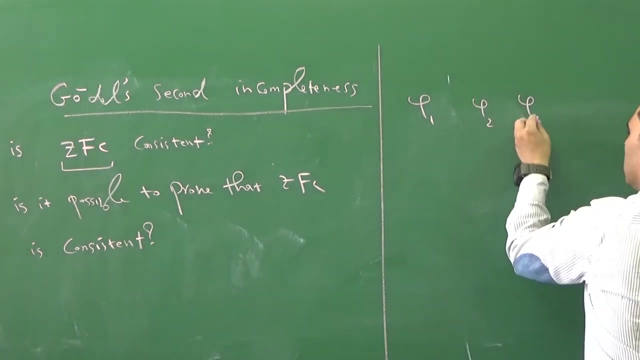 That is contradiction free, Alright, I'm just going to give a proof why that's not possible. Alright, So assume that I've listed all formulas in ZFC: Phi 1,, Phi 2,, Phi 3,, Phi 4.. 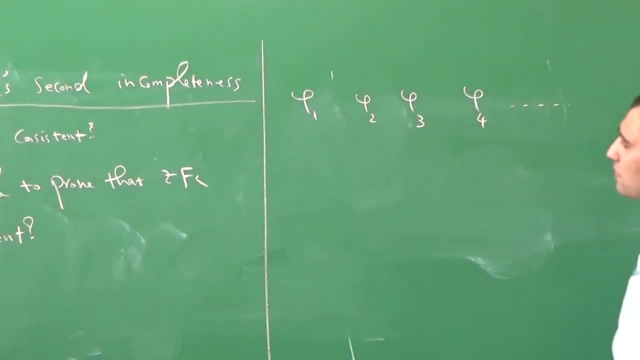 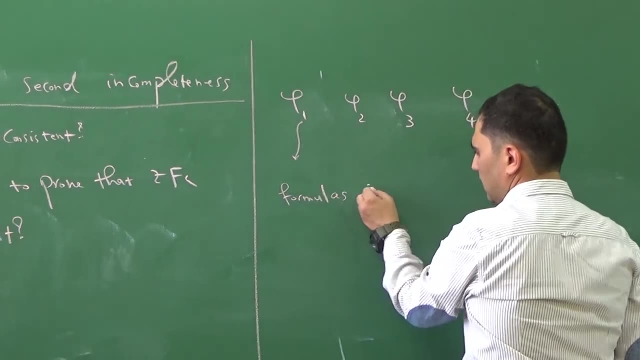 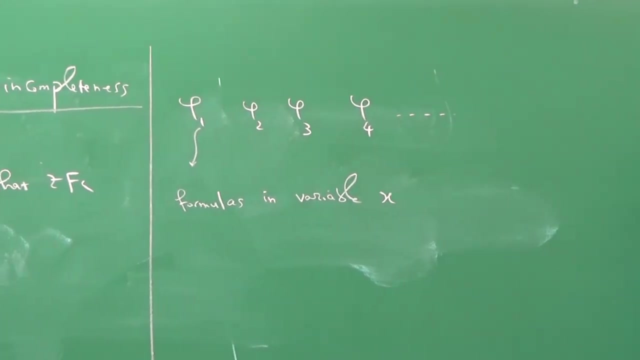 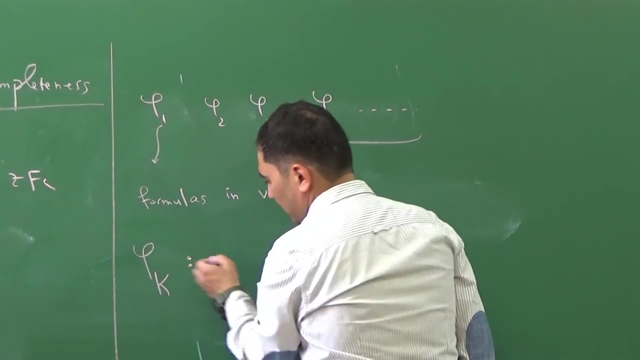 That's my list of all formulas. Actually, I'm listing formulas in one single variable, So these are formulas in the variable x. Quite interestingly, one of these formulas, for example 4k, is the formula that says this: 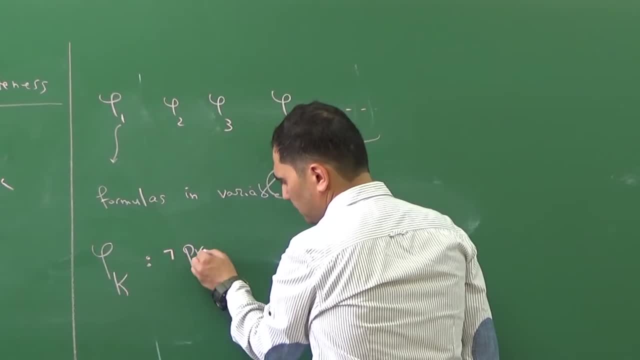 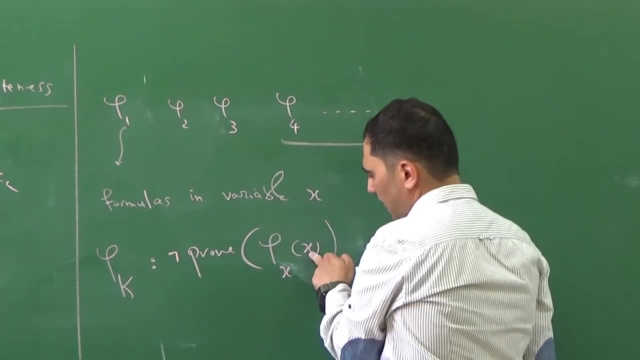 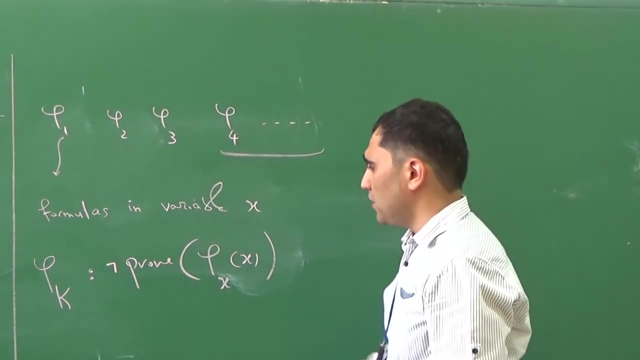 It says it's not possible to prove phi x of x. Phi x of x is when you put x in the formula with index x. Why is it possible to write such a formula? You know the concept of proving something in mathematics can be done. 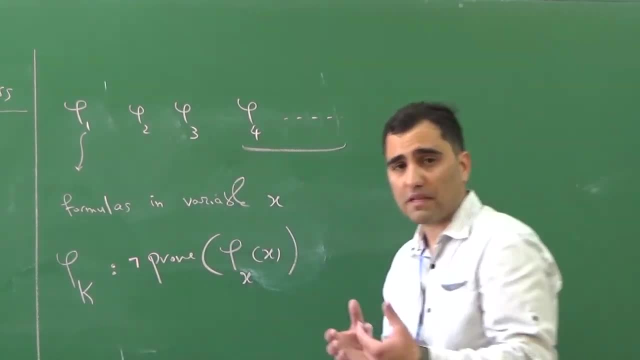 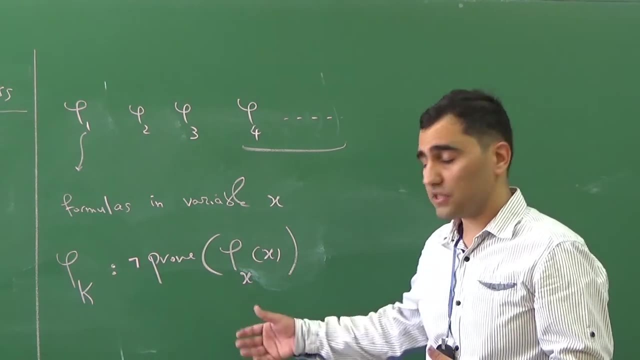 with an algorithm, So it's an algorithmic thing. Proofs in mathematics can be done using algorithms, And things that can be done with algorithms can be written with first-order formulas. So it's possible to write a formula that says this thing is not provable. 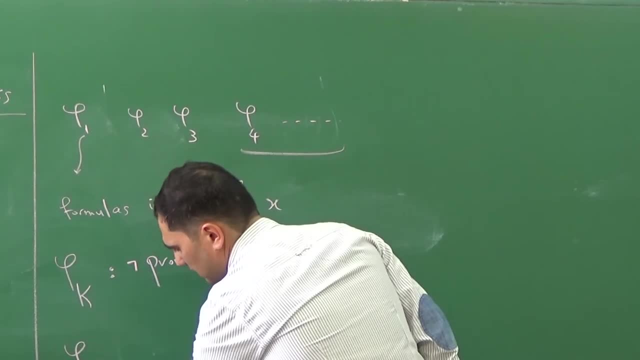 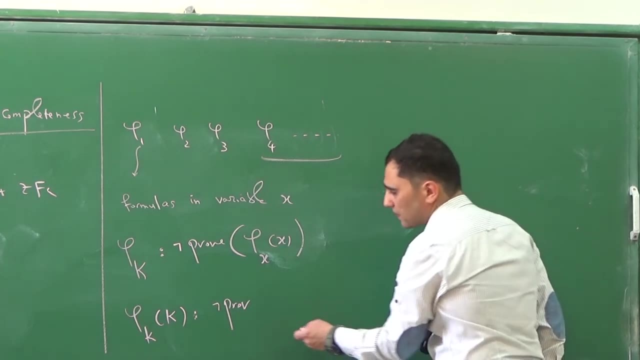 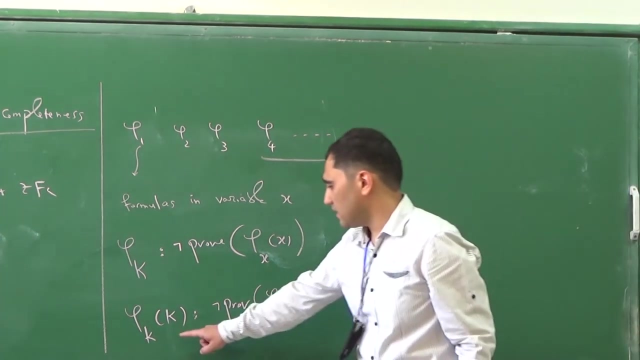 So what happens when I consider phi t of k? Phi t of k says it's not possible, there's no proof. there's no proof for phi k of k, And that's even more interesting because phi t of k says it's not possible. 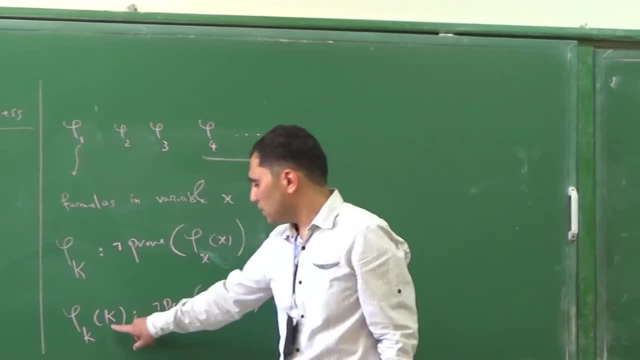 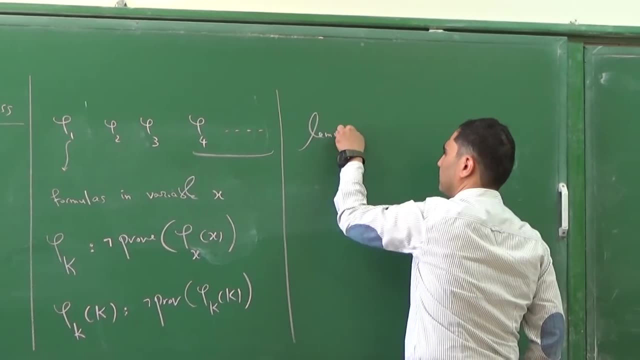 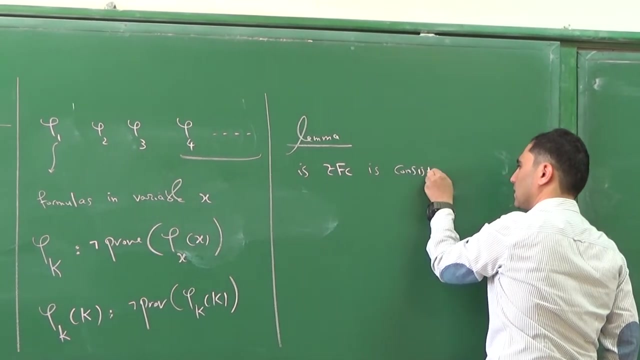 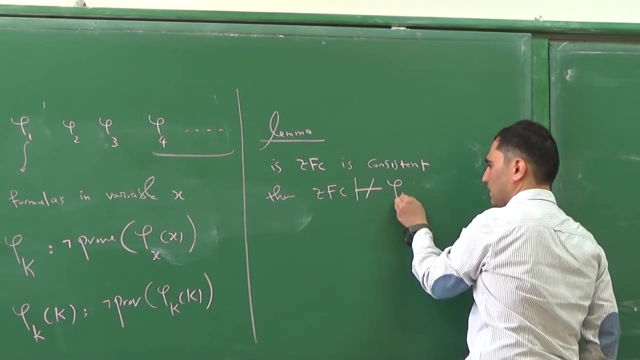 to prove v. So we have written a formula that says you cannot prove v. Alright, Okay, I have a lemma here. Lemma: If z of c is consistent, then it cannot prove phi k of k, Because if z of c proves, 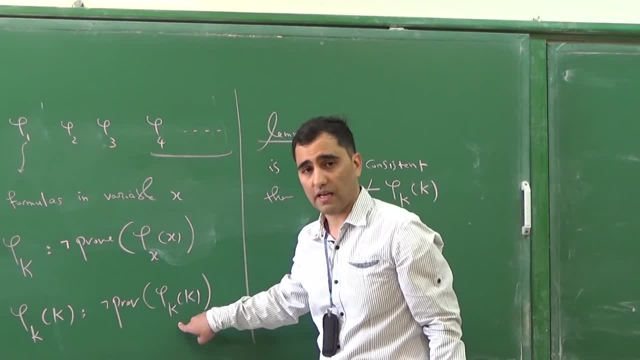 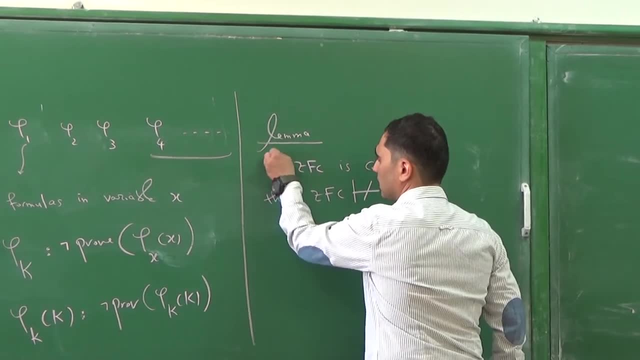 phi k of k, then it proves that it cannot prove phi k of k, And that would be a contradiction. So that's quite easy to prove that if z of c is consistent. sorry, that's an if. So if z of c is consistent, 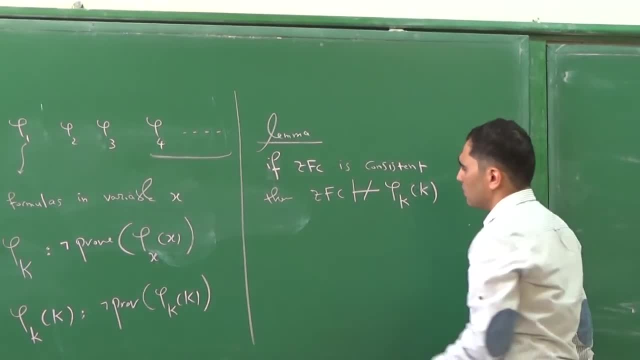 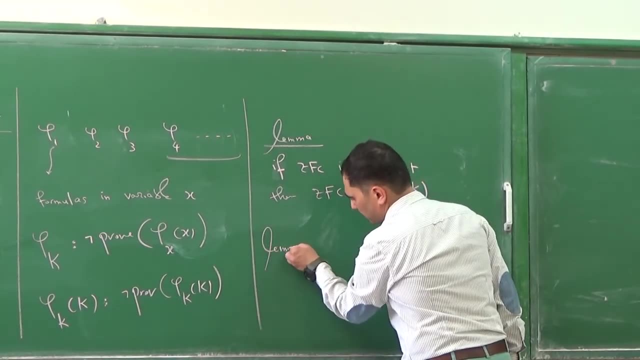 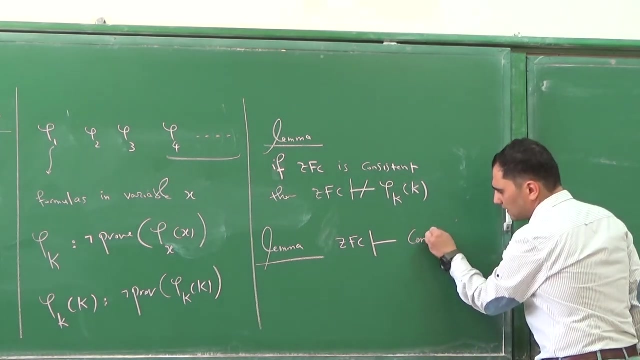 then it cannot prove phi k of k. So let me just write it this way: If z of c- okay, I'm just gonna rewrite this lemma as in the following lemma: In z of c, this happens If consistency of z of c. 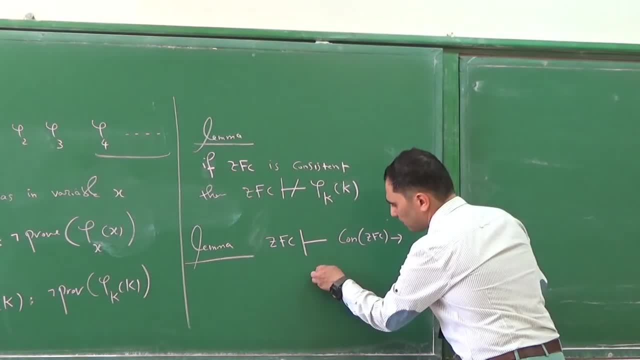 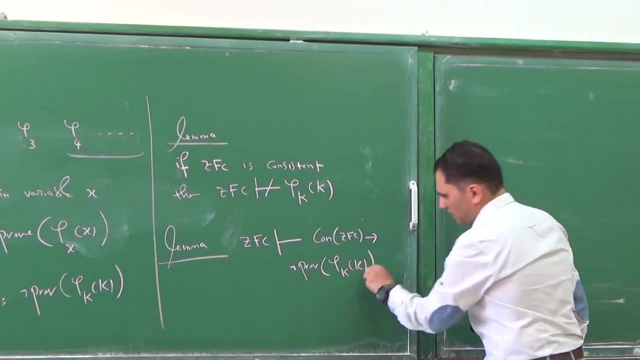 is consistent, then negation of, negation of. so you cannot prove phi k of k, But that's quite interesting, because negation of the probability of phi k of k is what phi k of k is about. Alright, You may ask me. 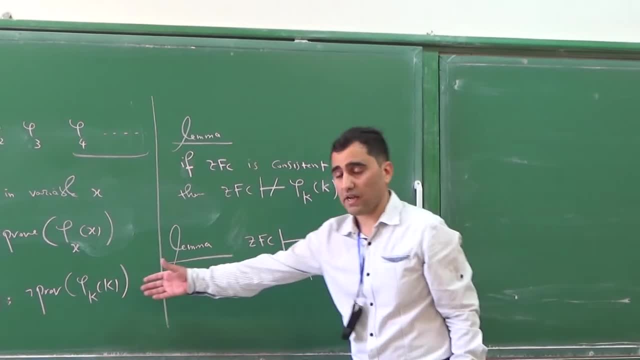 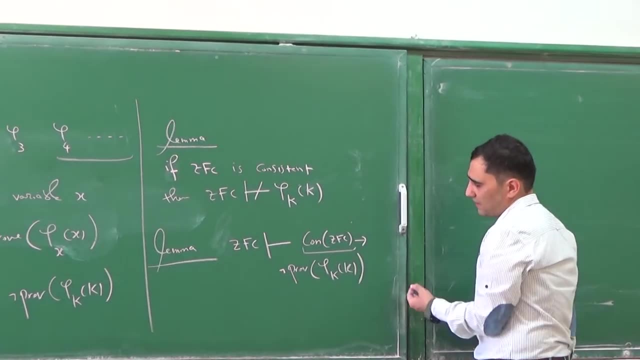 what does that mean? Consistency of z of c. So that's also a first order formula that says z of c is consistent. So it means that you cannot prove phi k of k if z of c is consistent. So if z of c. 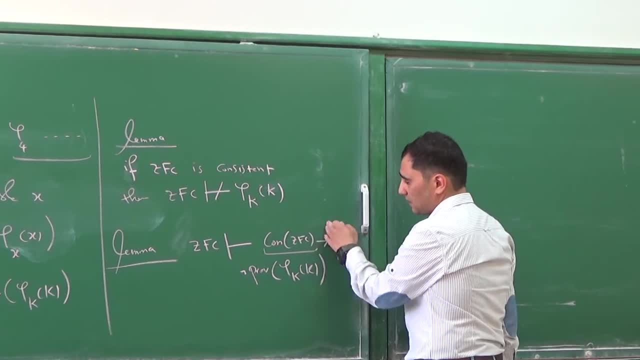 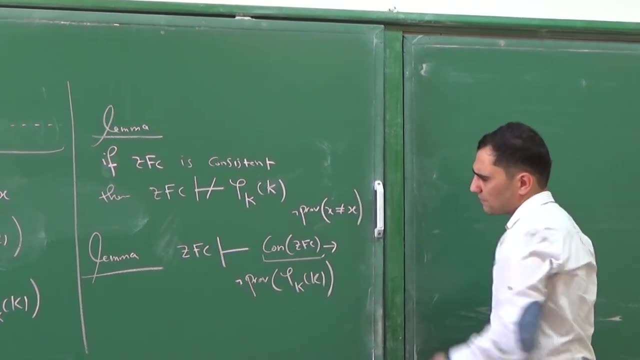 is consistent, then you cannot prove phi k of k if z of c is consistent. So some contradiction. for example, you can't prove that x is not equal to x, So it's possible to write a formula that says z of c is consistent.